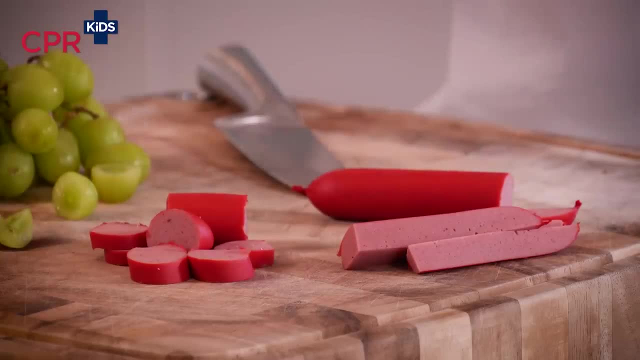 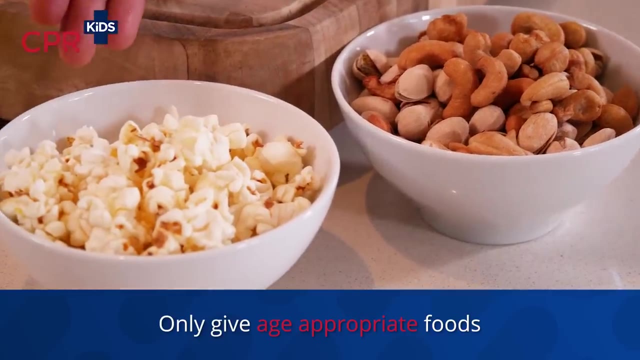 than to have that perfect circle lodged in their airway. Think about other types of foods as well. Young children shouldn't be eating whole nuts. Popcorn can be quite dangerous to lodge in an airway too. Perfectly fine for older kids, but be really cautious in the younger ones. 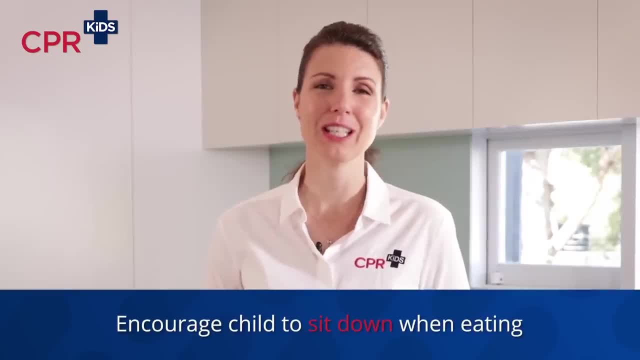 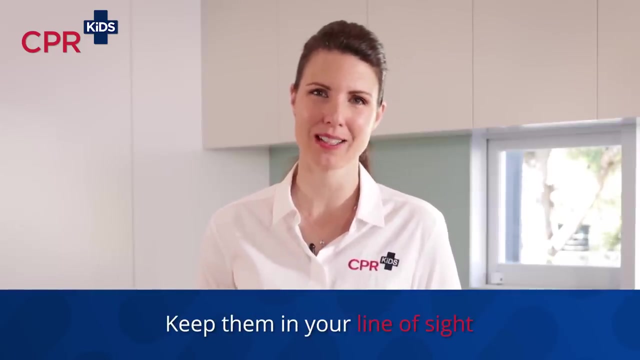 When it also comes to prevention, what I encourage you to do is get your children to sit down to eat- Children who run around with objects or food in their mouth are more likely to choke- And also make sure you keep young children in your direct line of sight. It can be really. 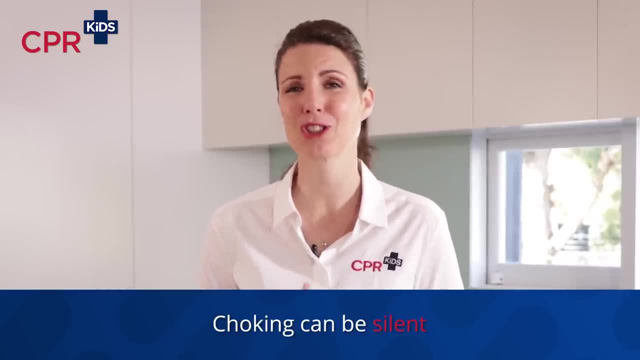 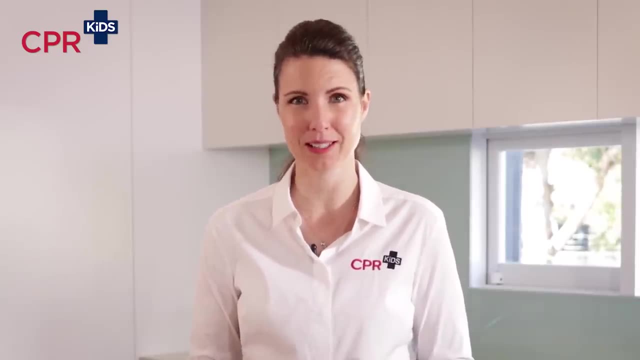 tempting just to nip off and have a quick shower while your child is settled in their high chair. But what's really important is that you remember that choking can be silent. Always keep young children in your line of sight, watching them while they're eating. 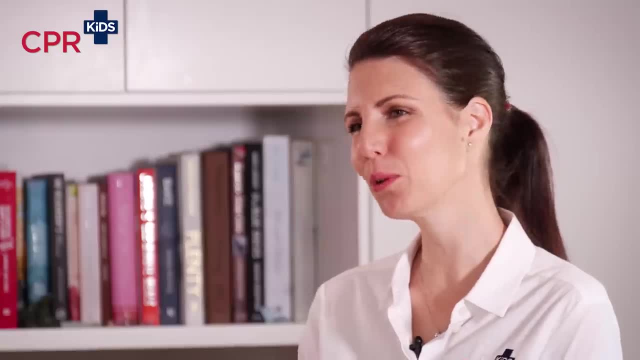 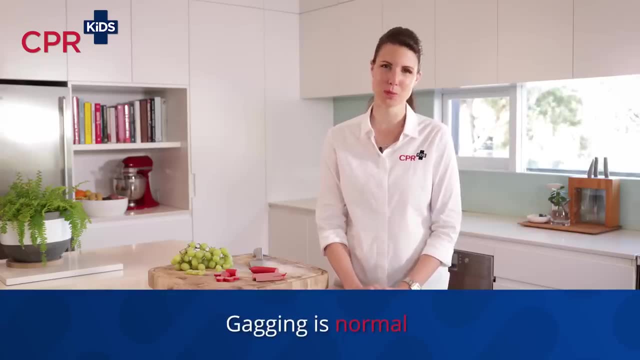 When it comes to recognising choking in children, it's really important to understand that choking is different to gagging. Gagging is a completely normal response. You may notice when you introduce solids to your child that you know the first little while when. 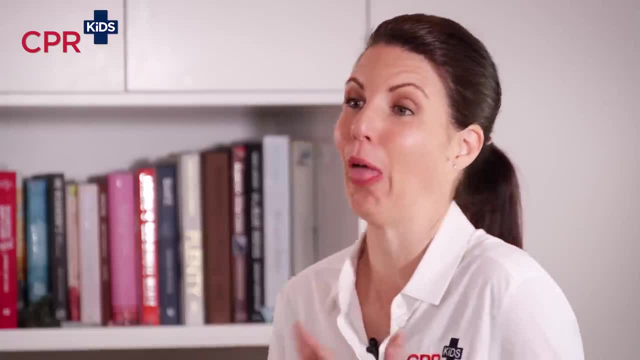 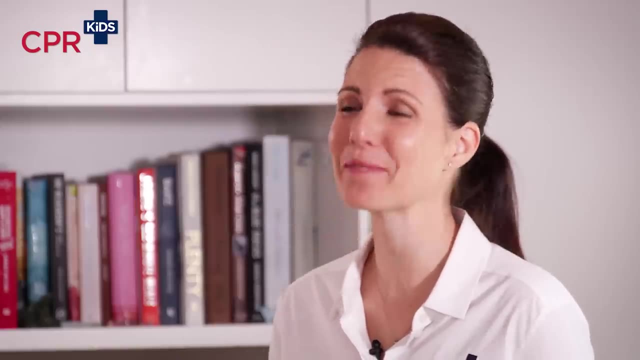 you're doing that. you'll pop a spoonful of food in their mouth and they will. they will gag, They will vomit that food up. They'll then pick it up again and start eating it again and it's disgusting, but it's completely. 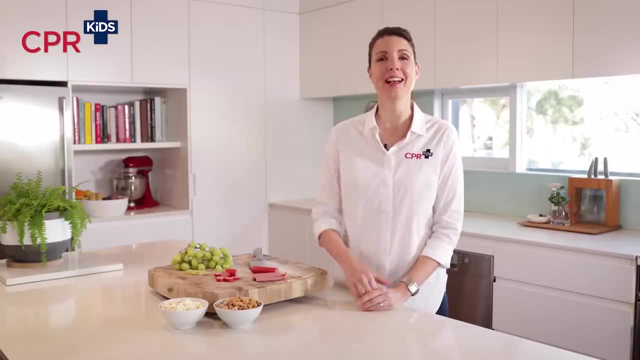 normal. So remember your child. when they gag, they may get a little bit red in the face, They may have watery eyes, They may cough, They may vomit that piece of food up, But they're not distressed and they're able to clear it themselves. 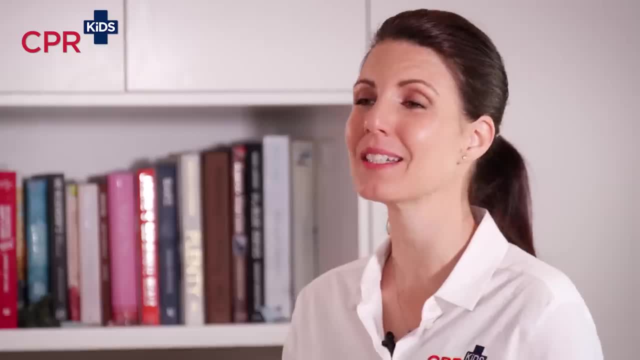 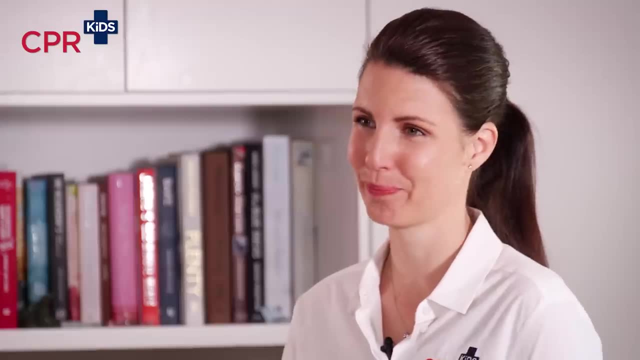 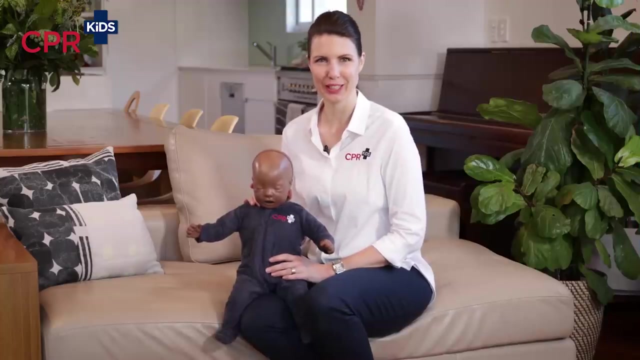 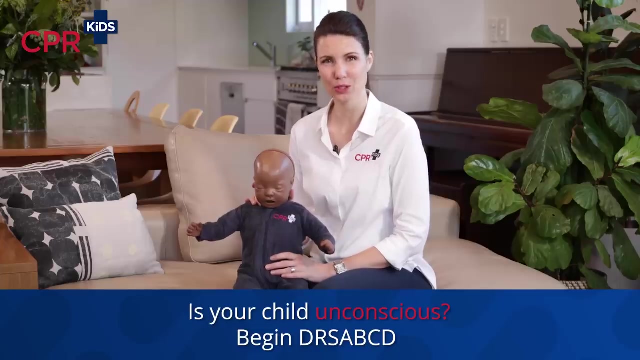 Choking is different. Choking is when something is lodged in their airway or oesophagus. They are in distress and we need to help them. If your child is choking, this is what you're going to do. Firstly, if they are unconscious, you need to go through doctors, ABCD. 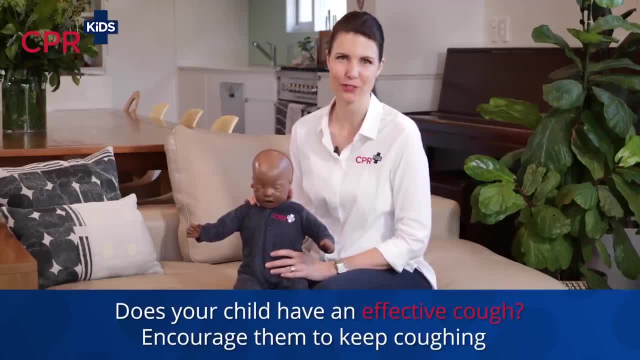 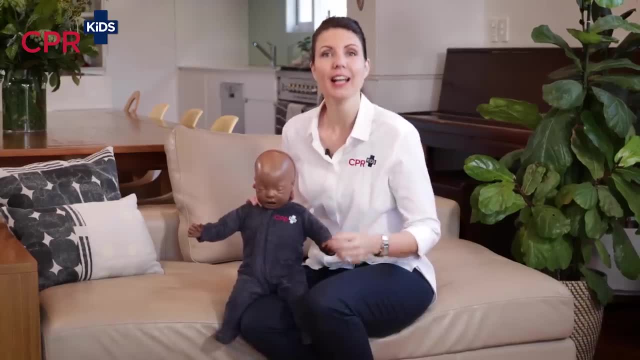 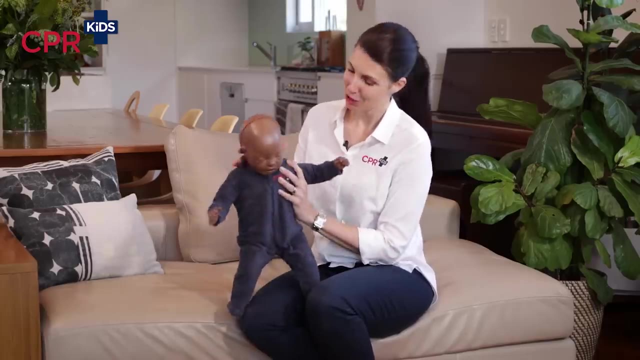 If your child has what we call a strong, effective cough, that is, they're able to take a big breath in and a big cough out, Then what you're going to do is encourage them to keep coughing. Now you may be tempted to go and stick your fingers in your child's mouth and try and 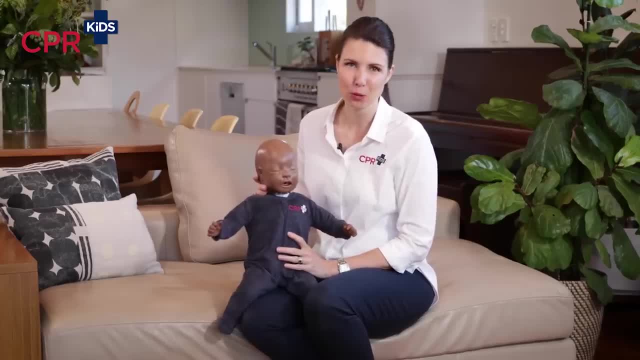 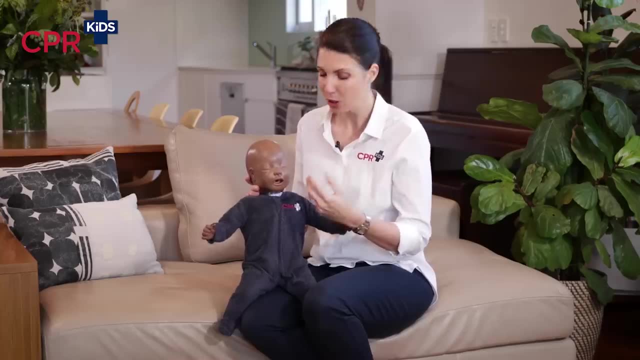 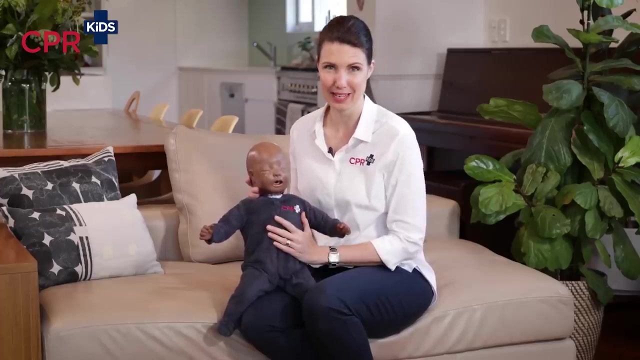 dig out whatever is in there. Please be cautious, because if you do this, you may push that object further down. If the object is at the front of the mouth and you can easily remove it, please do so. Otherwise leave it there. 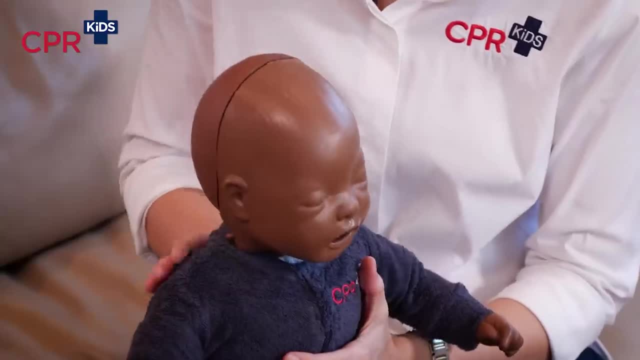 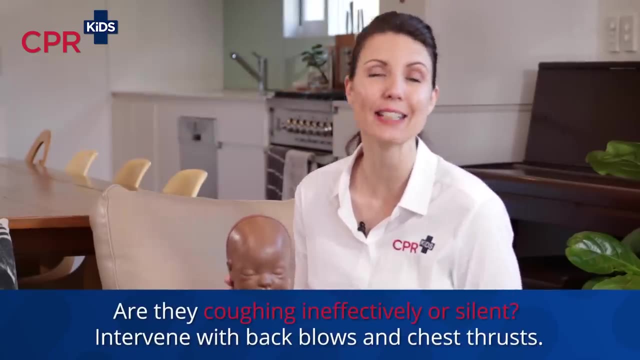 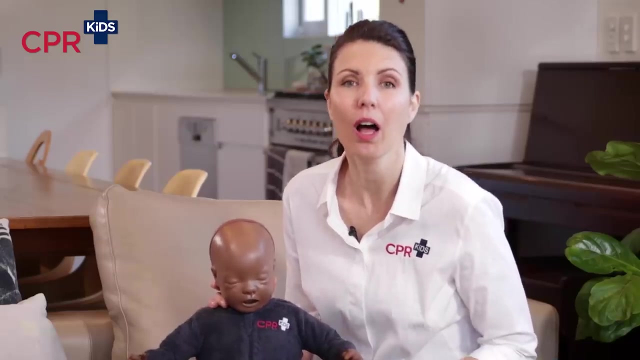 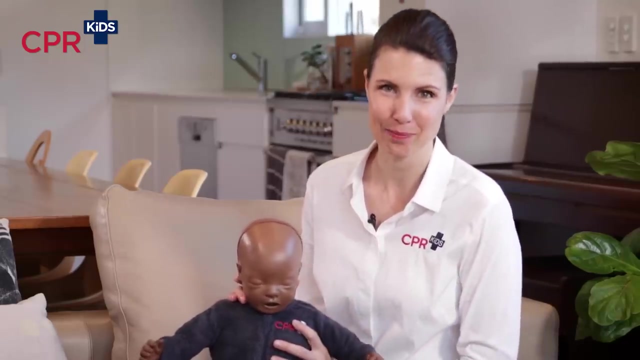 If their cough is strong and effective, simply encourage them to keep coughing and watch them closely. If your child has an ineffective cough, or they're silent, so they are, or that's not a strong lungful of air in or out, then we need to intervene. 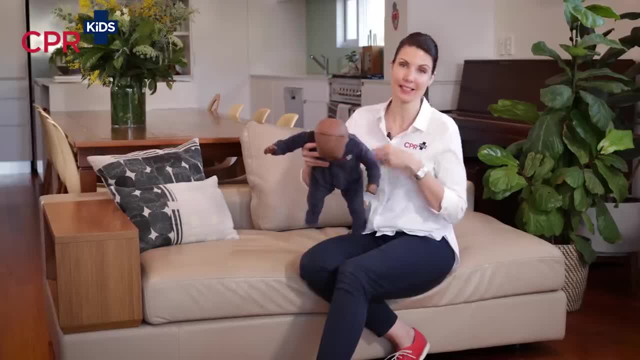 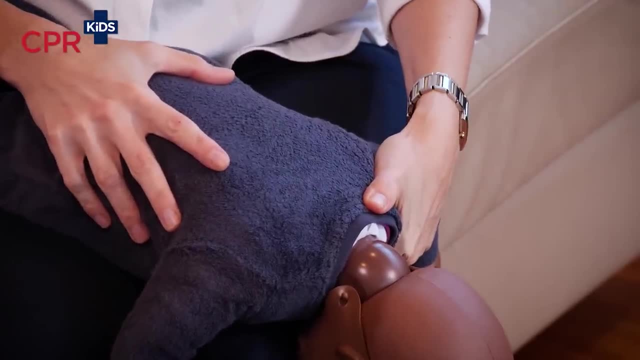 We're going to take the baby out of the high chair, or whatever it is that they're in. We're going to lay them down across our laps, Hold them so that you're not going to drop them. Ideally, we want their bottom higher than their head. 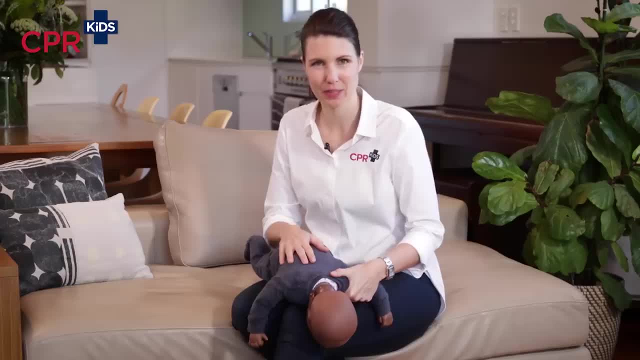 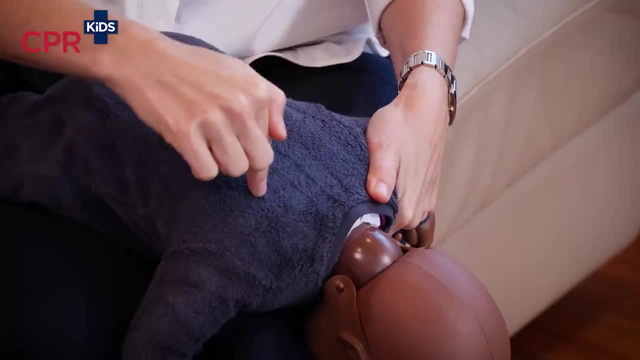 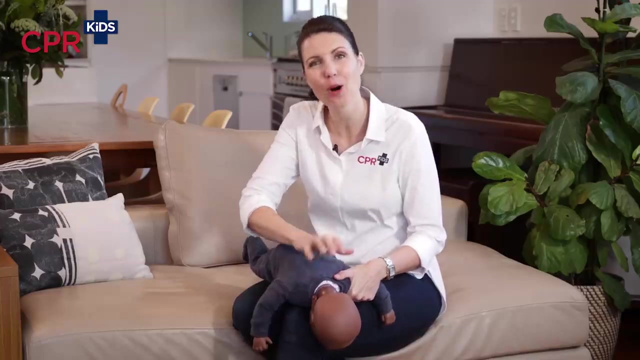 And we're going to give back blows and chest thrusts. A back blow is not a whack on the back using the heel of your hand between their shoulder blades. It is a firm blow to expel the air out of their lungs to try and pop that object out. 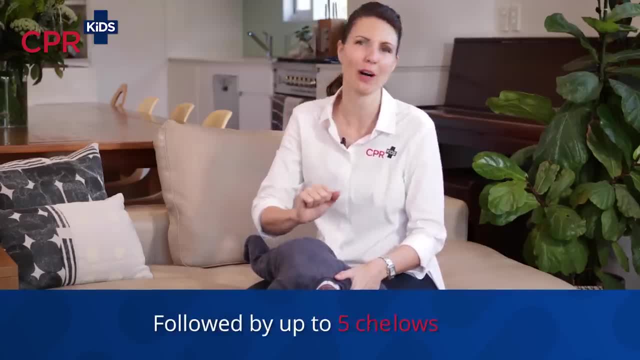 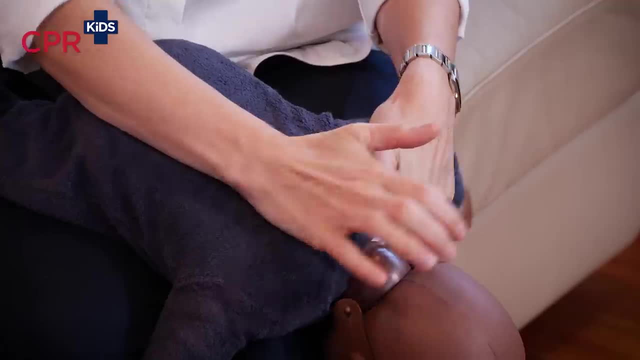 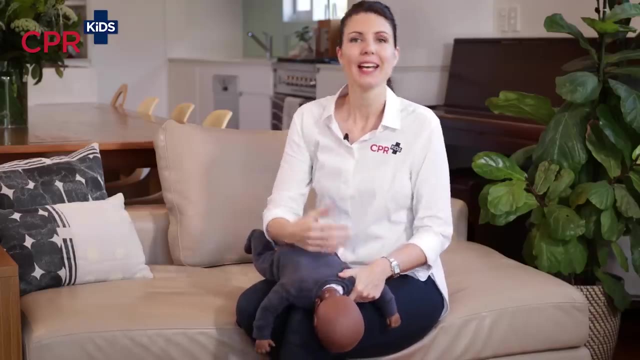 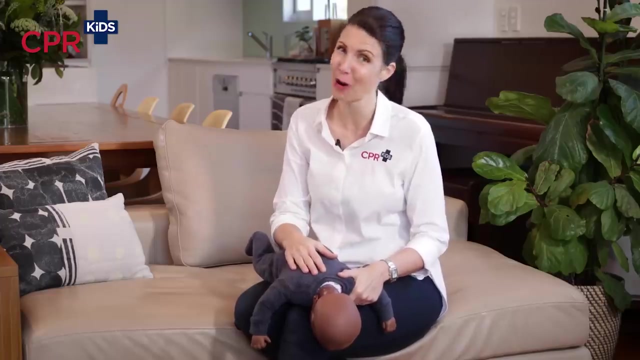 We can give up to five back blows followed by up to five chest thrusts. So one, two, three, four, five, Checking after each blow to see if the object has come out. If the object comes out after the first one, you don't need to give all five. 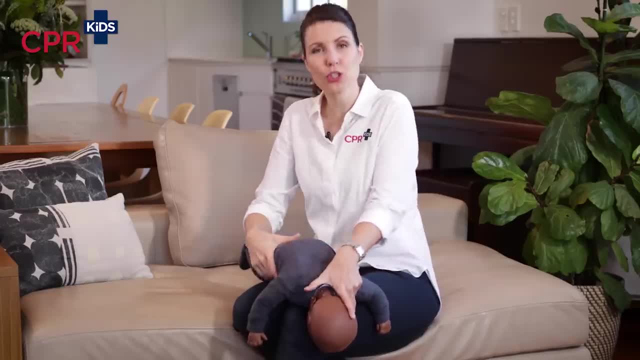 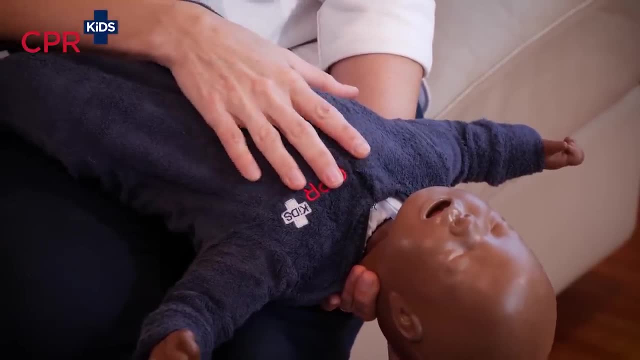 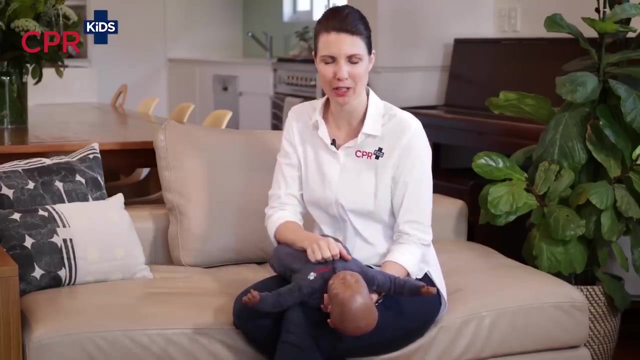 If the object has not come out, turn your chest out, Turn your child over Once again, bottom higher than their head, and holding them firmly, We're going to give chest thrusts. Two fingers for a small baby, Heel of your hand for a bigger baby or child.